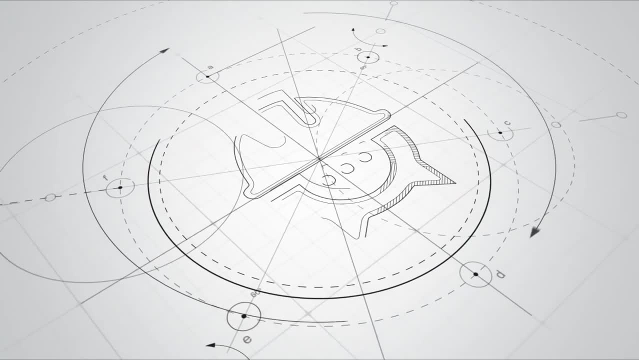 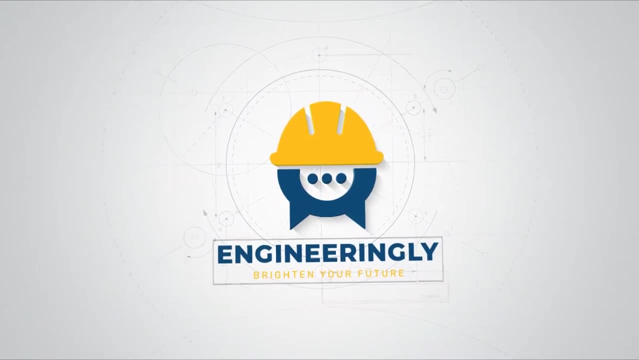 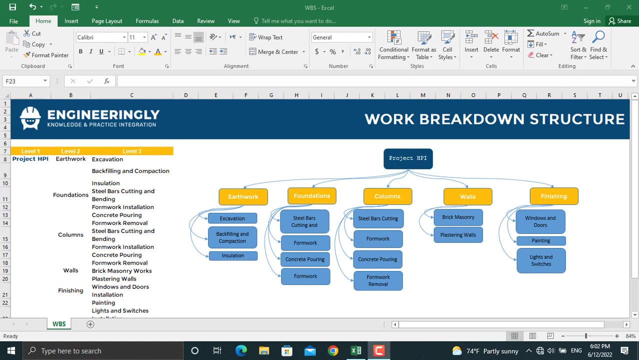 Hi, in today's video we will talk about WBS and project management. It's a hierarchical outline of the tasks required to complete a project. The WBS decomposes the structure of a project into manageable deliverables. Using the WBS, you decompose your project into smaller components In more complicated 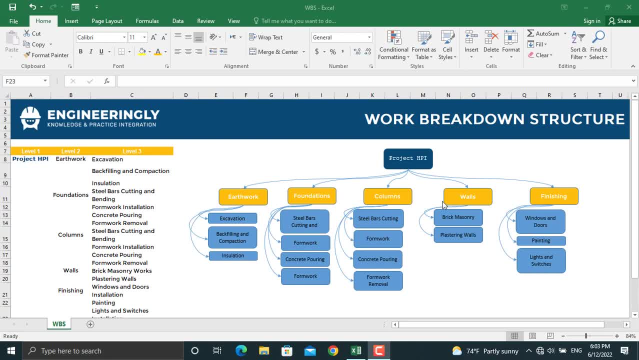 projects, the WBS might not look this simple, As you can see for the project HPI, at level 1 we have the project name and the level 2 we have decomposed the project into elements of the building, which are the foundations, columns, walls. 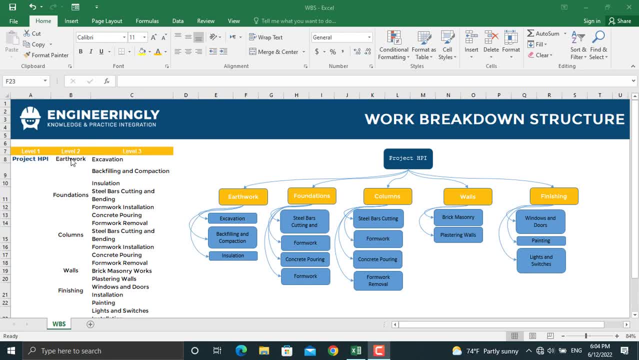 and finishing. Furthermore, in level 3, the earthwork and all the other elements are decomposed to activities. In this video, I am going to show you how to prepare a WBS using Microsoft Excel. Organizations and companies might use different methods for preparing their WBS, but this is the most conventional. 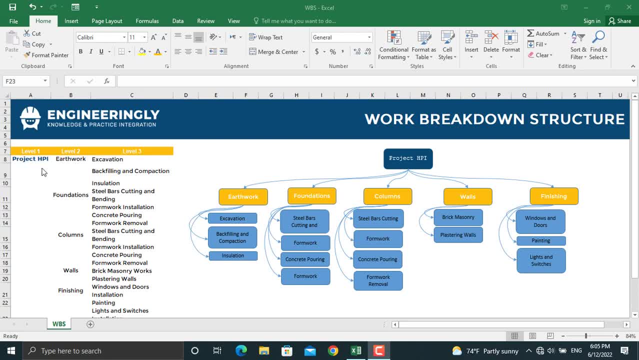 method and the most easy to understand. In the level 1, you write down the major deliverables of the project or the project itself. Then, at level 2, you decompose the deliverables into work packages. Later on, in the lower levels, you decompose the work packages into activities. Now, in order to create the 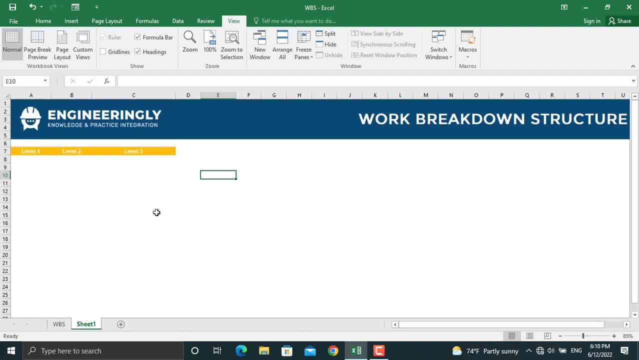 WBS. we will carry out listing the deliverables and preparing the diagram at the same time. First of all, let's insert the shape that we want for our WBS. I'll select this one, I'll draw the shape here and then I will link the 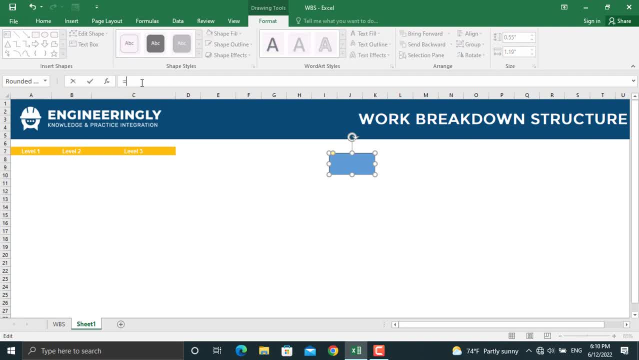 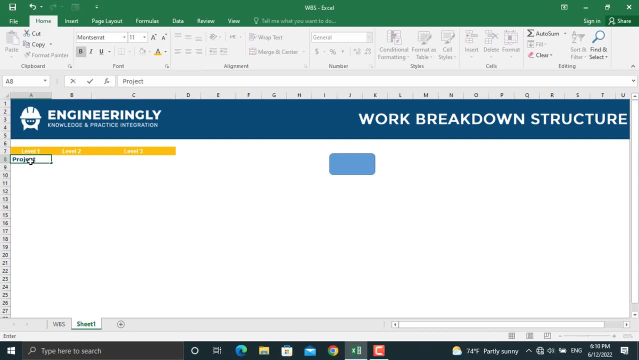 shape to the project name. I will write down equal sign here and I will select the cell Now in here I will write down project HPI. As I press ENTER, the name will appear in here as well. Next thing is to write down the major deliverables. 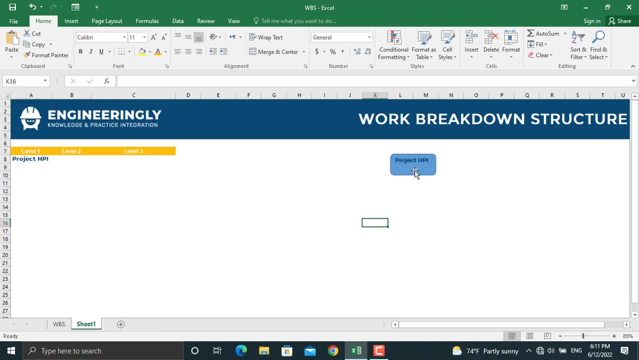 under this project. Now I will write down the major deliverables under this project. Now I will write down the major deliverables under this project. Now I will copy this shape and paste it here as a deliverable of the project. But the only difference is that I will link this to a cell in level 2.. This cell In this 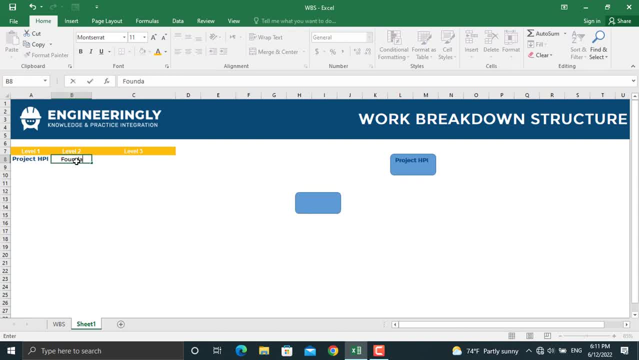 cell. I will write down the foundation Again. I am going to copy this and we'll leave it here. We will write down columns. Furthermore, I will link this shape to the column cell. So in here I'll remove this and click this cell. Our next element in the project will 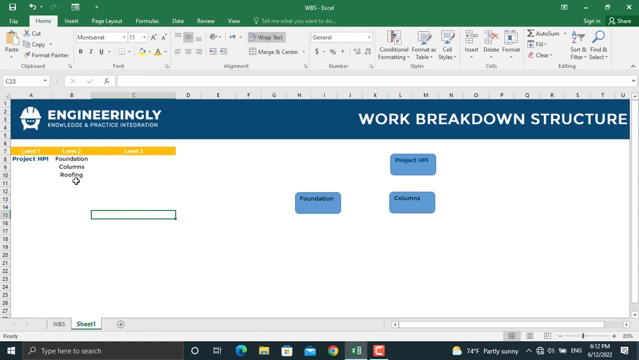 be roofing, Where the beams and slabs and everything comes For this one. I will copy this shape and paste it here. Now. I will copy this shape and paste it here, Drag it to the right here. I will link this shape to its associated cell. Next thing: 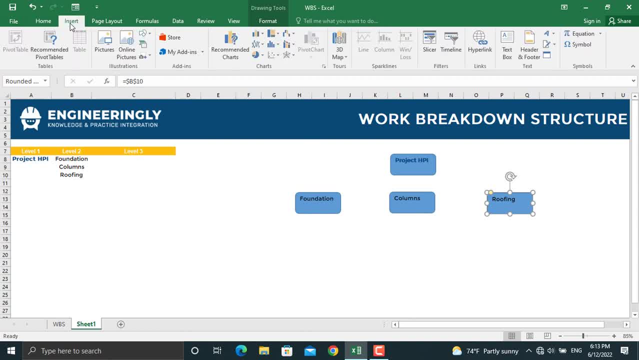 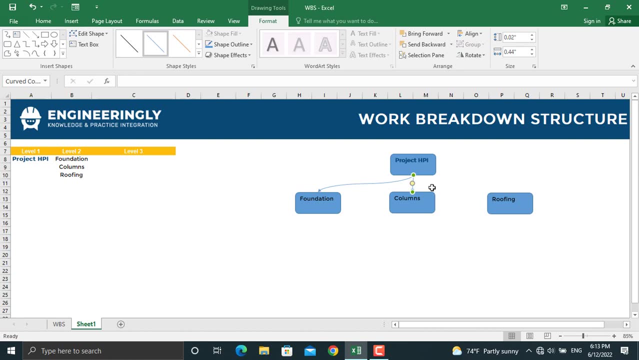 is to connect the shapes, Go to insert and from there we will select an arrow and we will connect each of these. I will copy this arrow and paste it. I will connect it to columns And I will do the same for the roofing. I will click on this arrow and paste it. I will 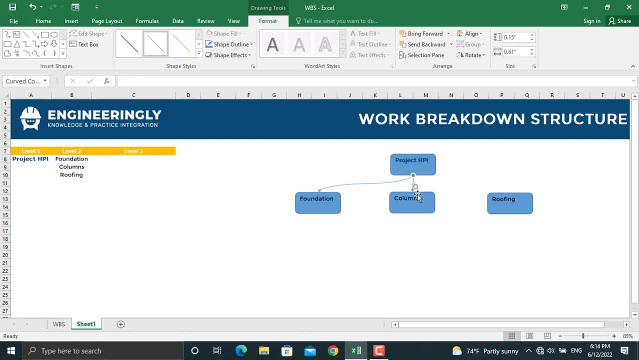 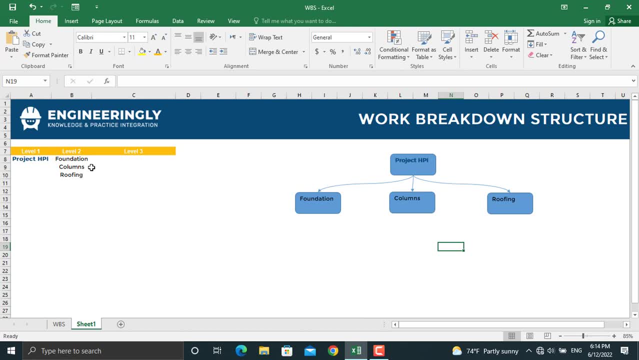 same for the roofing. I'll connect it to both ends. now let's further break down these deliverables into activities. for example, for the foundation, let's assume we have two activities. activity number one for the foundation will be the earthwork and activity number two will be the concrete works. 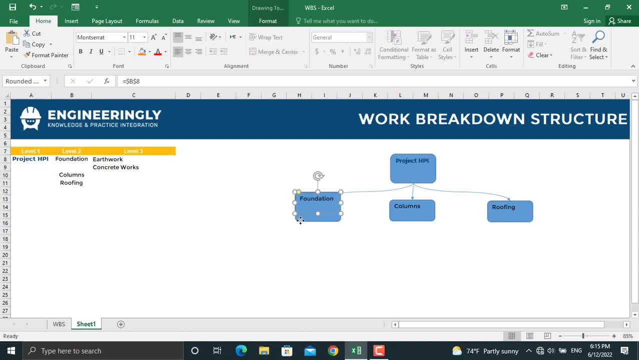 now under the foundation. I will copy this shape and paste it. I will take another copy from this one and then I will link them to their selves. this one should be linked to the earthwork cell and the next one should be linked to concrete work. so I will copy the arrows and connect the foundation. deliverable.